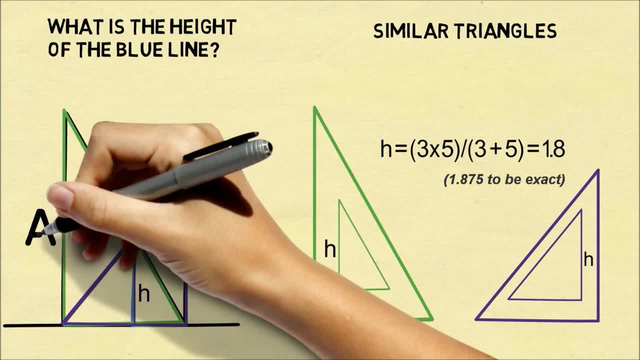 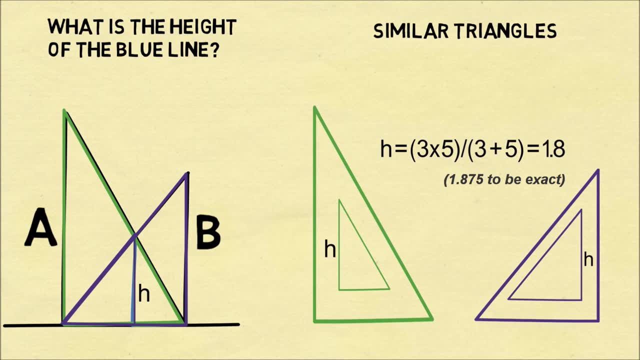 So that's pretty neat. We can figure out the height of the blue line just from the distances of the two walls. Now let's generalize the problem. Imagine one wall has a length of a, another has a length of b. We can go through the same steps and we can conclude the height is equal to a times b over a plus b. 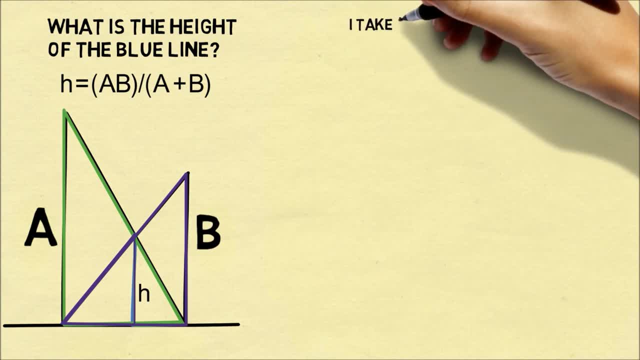 And this is interesting- it doesn't depend on the distance between the walls. Now let's consider another problem. Imagine I take a hours to do a job and you take b hours to do the same job. How long will it take if we work together? This is a totally different problem. 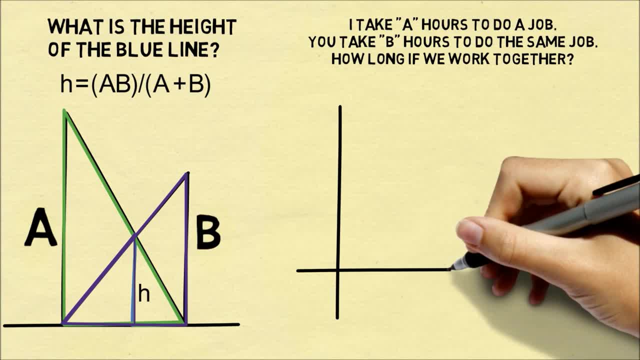 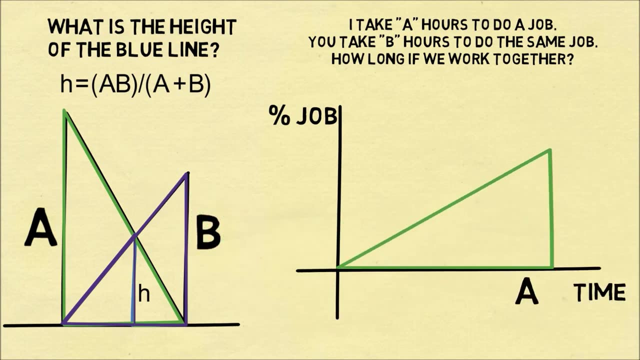 but I'm going to show you how these two problems are related. So let's draw a graph where the horizontal axis is time and the vertical axis is the percentage of the wall. The horizontal axis is the percentage of the job completed. If I do a job in a hours, that means it will take me a hours to get a hundred percent of the job done. 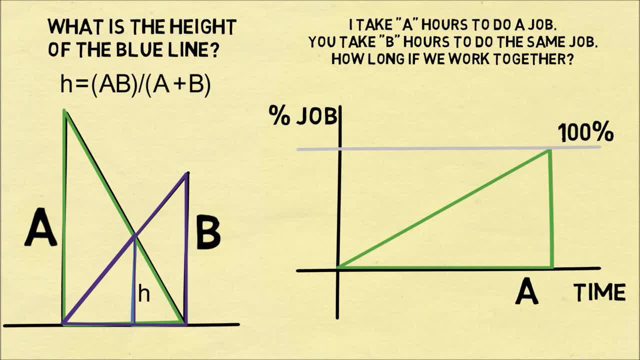 and I will linearly increase the percentage of the job from zero to a hours. If you take b hours to do a job, that means you will complete the job in b hours, going from zero to a hundred percent of the job completed. So let's imagine we're working together and we're going to do a little trick. 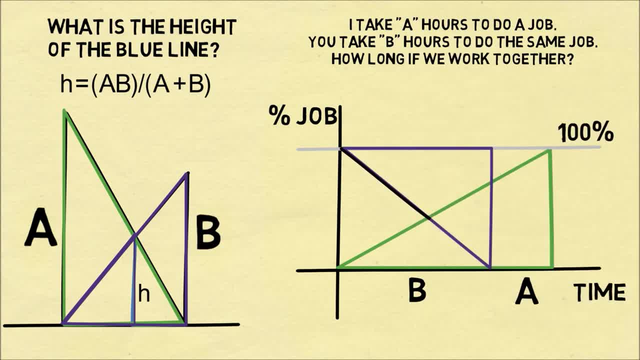 We'll flip the triangle and now imagine that you are working from the end of the job and I'm working from the beginning. The point at which we cross is the amount of time it'll take us to work together, and that's the blue distance If I translate over the purple triangle and I move over. 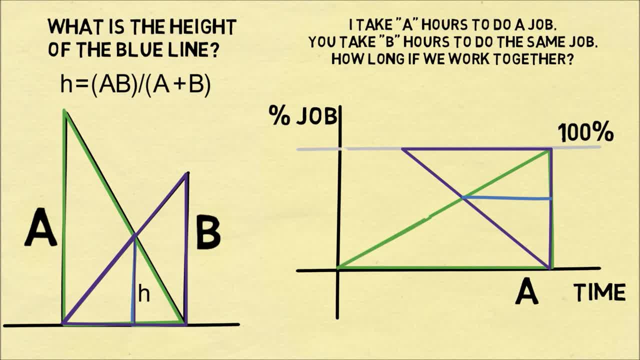 this blue distance. you'll exactly see that this blue distance is the amount that we're working together, and the geometry is exactly the same as the previous problem we've just solved. therefore, we can conclude: the time it takes to work together is the same amount a times b divided by a plus b, and that's pretty neat. 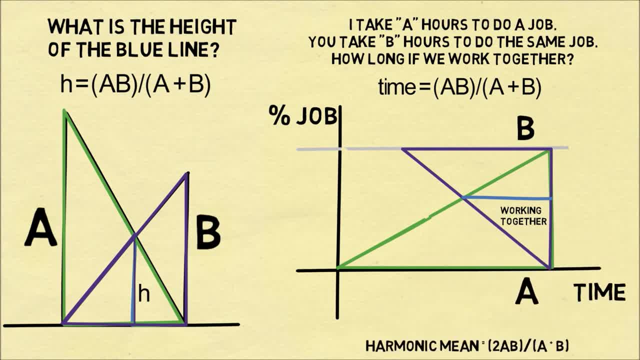 these two problems are related. on a concluding note, the harmonic mean is equal to two times a, b over a plus b, and both of these problems are equal to half of the harmonic mean. please subscribe to my channel. you can support me on patreon. catch me on my blog. mind your decisions.